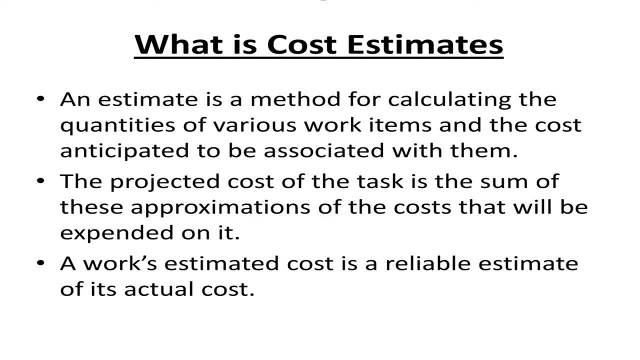 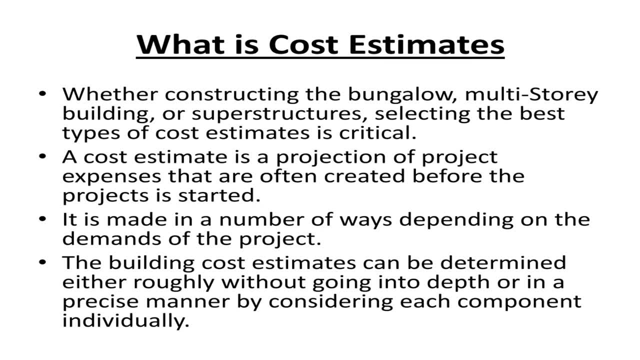 Is the sum of these approximations Of the costs That will be expended on it. A work's estimated cost Is a reliable estimate of its Actual cost, Whether constructing the bungalow, Multi-story building Or superstructures. Selecting the best types of cost estimates Is critical. A cost 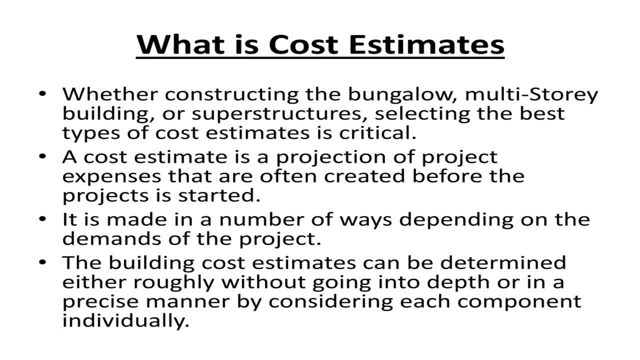 estimate Is a projection of project expenses That are often created Before the projects is started. It is made In a number of ways, Depending on the demands Of the project. The building cost estimates Can be determined either Roughly, without going into 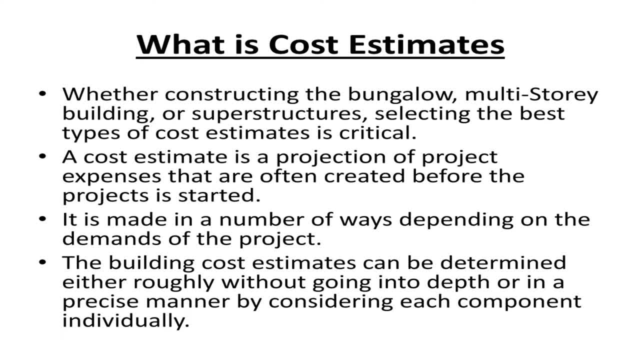 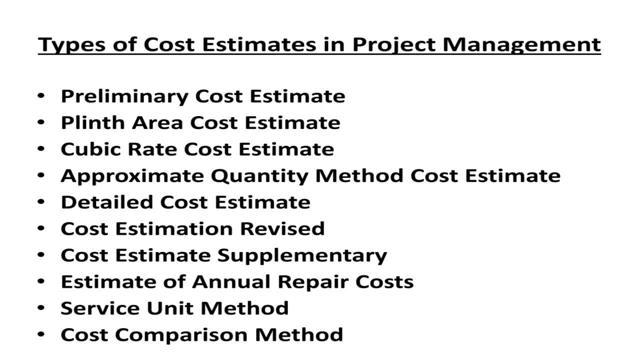 depth Or in a precise manner, By considering each component individually. Types of cost estimates in project management: Preliminary cost estimate: Plinth area cost estimate. Cubic rate cost estimate. Approximate quantity: method cost estimate. Detailed cost estimate: Cost estimation. 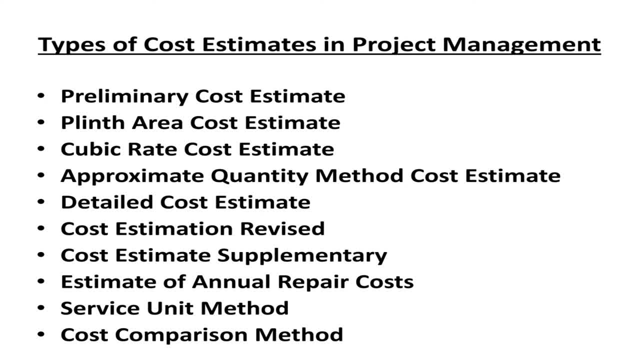 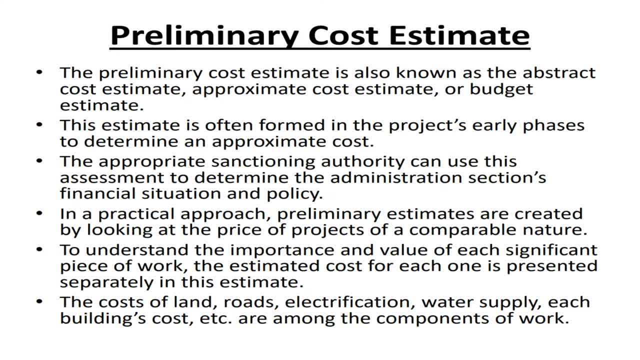 revised Cost estimate. supplementary Estimate of annual repair costs. Service unit method. Cost comparison method. Preliminary cost estimate. The preliminary cost estimate Is also known as The abstract cost estimate, Approximate cost estimate Or budget estimate. This estimate. 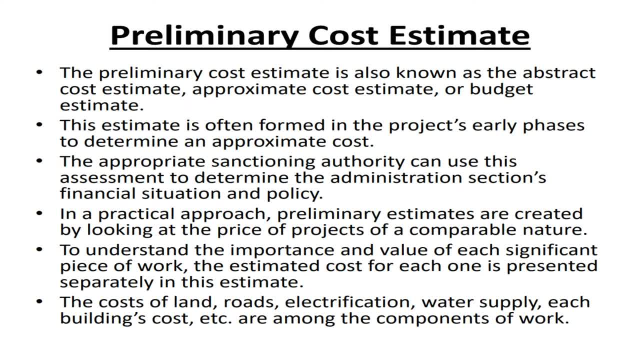 Is often formed in the project's early phases. To determine an approximate cost. The appropriate sanctioning authority Can use this assessment To determine the administration sections, Financial situation And policy In a practical approach. Preliminary estimates Created by looking at the price of projects Of a comparable nature To understand the importance 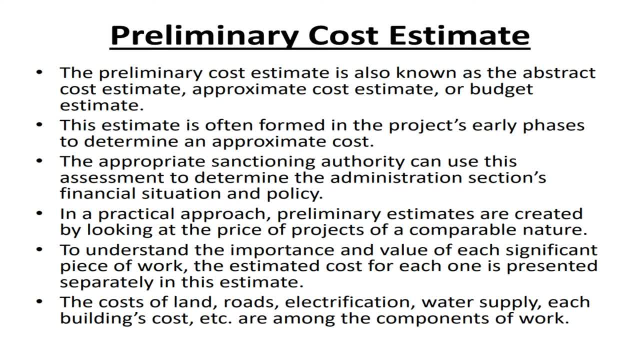 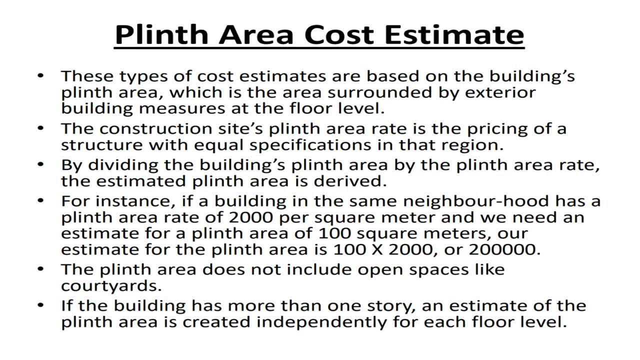 And value of each significant piece of work. The estimated cost for each one Is presented separately in this estimate. The costs of land, Roads, Electrification, Water supply, Each building's cost, Etc. Are Among the components of work. Plinth area cost estimate. 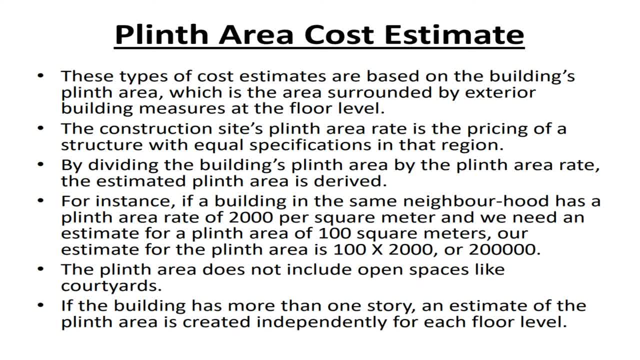 These types of cost estimates Are based on the building's plinth area, Which is the area surrounded By exterior building measures At the floor level, The construction sites Plinth area rate Is the pricing of a structure with equal specifications In that region By dividing the building's plinth. 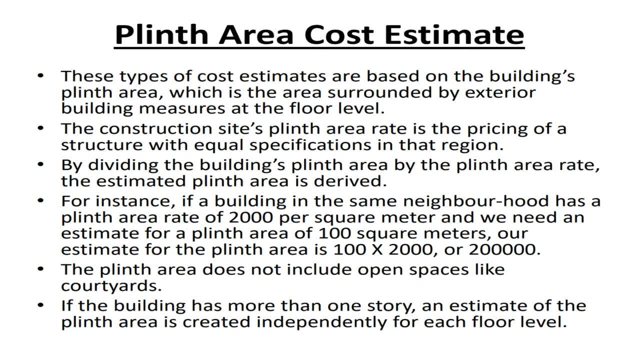 area By the plinth area rate. The estimated plinth area is derived. For instance, If a building in the same neighborhood Has a plinth area rate of 2000 per square meter And we need an estimate For a plinth area of 100 square meters, Our estimate for the plinth area is: 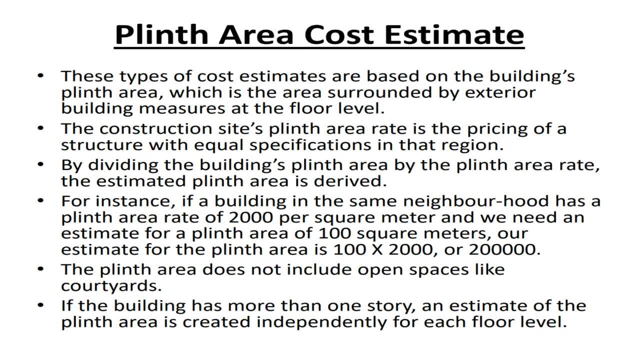 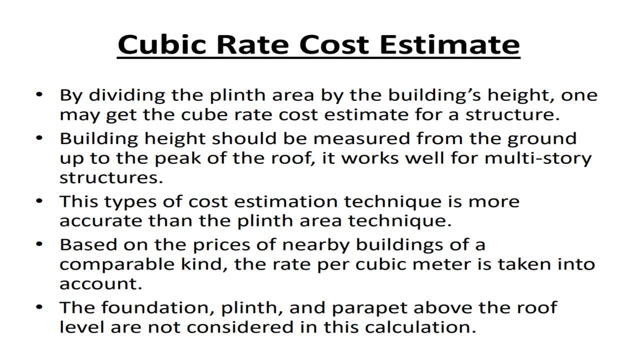 To lack The plinth area Does not include open spaces Like courtyards. If the building Has more than one story, An estimate of the plinth area is created independently For each floor level Cubic rate cost estimate. By dividing the plinth area By the building's height, One may get the 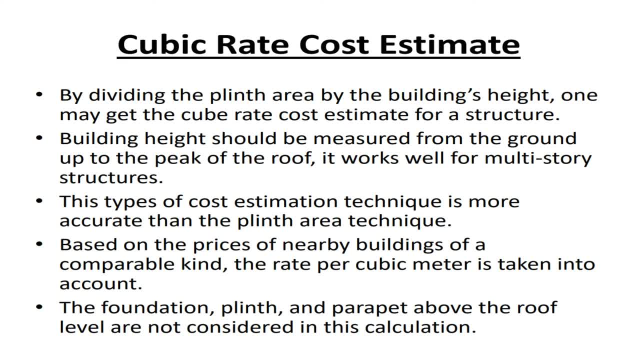 cube rate. cost estimate For a structure. Building height should be measured From the ground up to the peak of the roof. It works well for multi-story structures. This types of cost Estimation technique Is more accurate Than the plinth area technique Based on the prices. 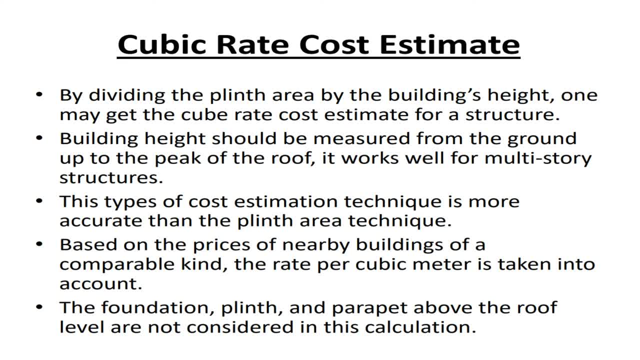 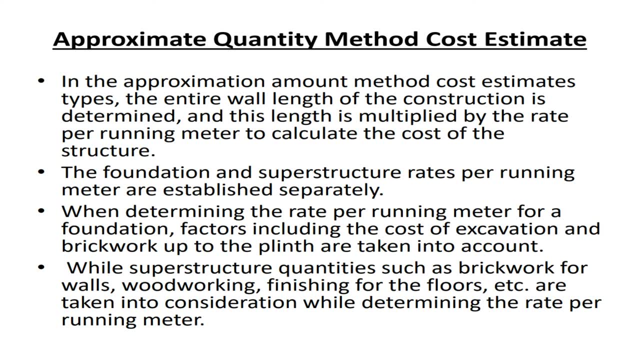 Of nearby buildings of a comparable kind, The rate per cubic meter Is taken into account. The foundation, Plinth And parapet Above the roof level are not considered In this calculation. Approximate quantity method: cost estimate In the approximation amount method: Cost estimates: types. 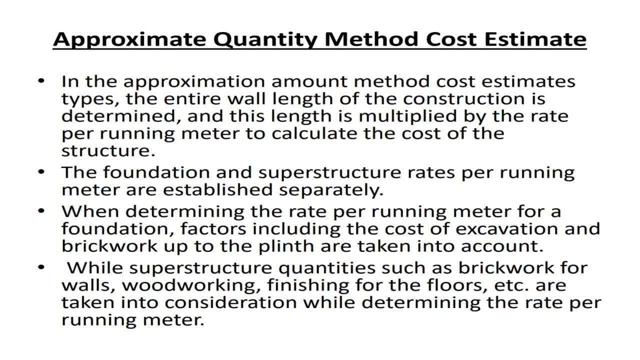 The entire wall length Of the construction is determined And this length is multiplied By the rate per running meter To calculate the cost of the structure. The foundation And superstructure rates per running meter Are established separately When determining The 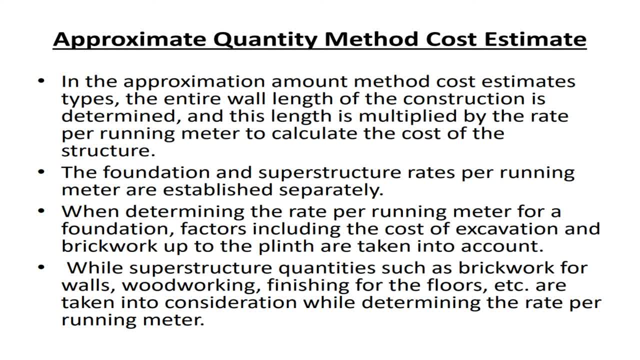 rate per running meter For a foundation, Factors, including the cost of excavation And brickwork up to the plinth, Are taken into account, While superstructure quantities Such as brickwork for walls, Woodworking, Finishing for the floors, Etc. Are Taken into consideration, While the 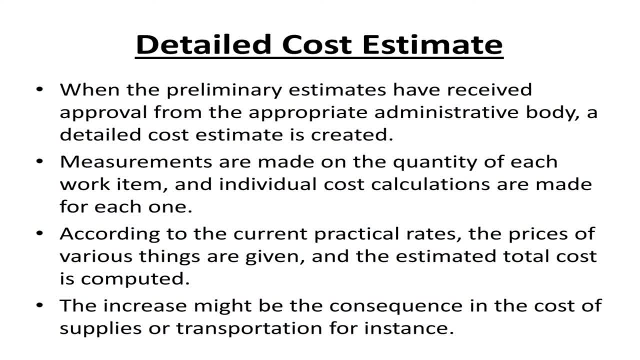 construction is done. The construction is done By determining the rate per running meter. Detailed cost estimate. When the preliminary estimates Have received approval from the appropriate administrative body, A detailed cost estimate is created. Measurements are made On the quantity of each work item And individual cost calculations Are made for each one According. 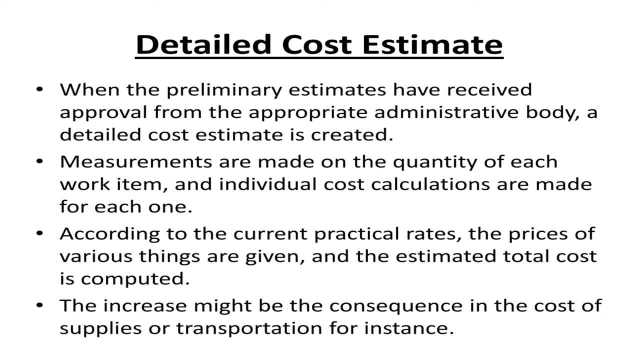 to the current practical rates. The prices of various things are given And the estimated total cost is computed. The increase might be the Consequence in the cost of supplies Or transportation, Or the cost of the construction, Or the cost of the construction Or the cost of. 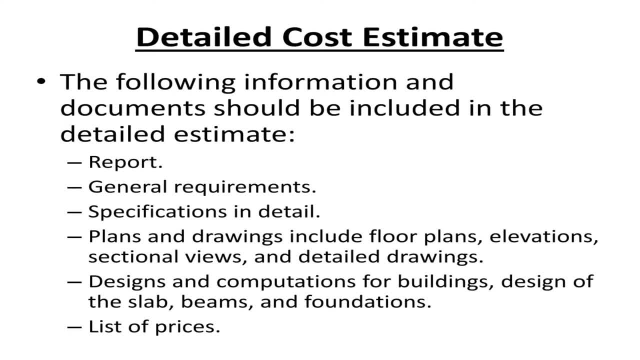 a building. Check out Junior LabSuncom. The following information And documents should be included In the detailed estimate Report: General requirements, Specifications in detail. Plans and drawings include floor plans, Elevations, Sectional views And detailed drawings, Designs And computations for buildings. Design of the slab. 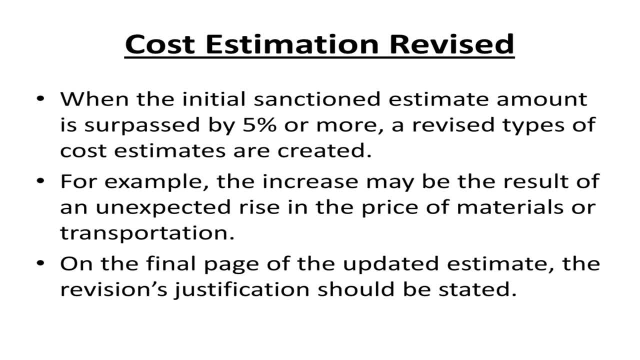 Beams And foundations. List of prices. Cost estimation revised. When the initial sanctioned amount has surpassed by 5% or more, a revised types of cost estimates are created. For example, the increase may be the result of an unexpected rise in the price of materials. 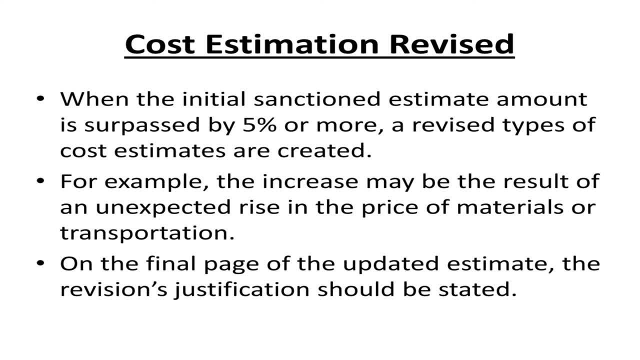 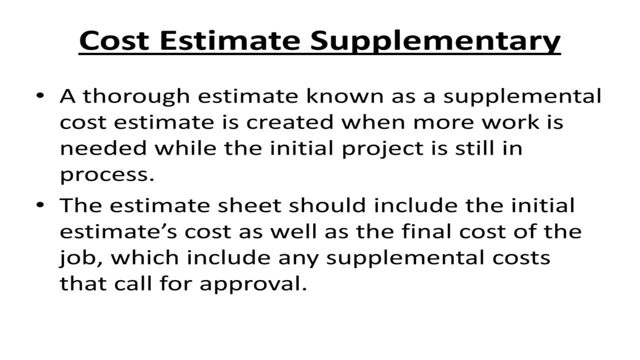 or transportation. On the final page of the updated estimate, the revision's justification should be stated: Cost estimate supplementary. a thorough estimate, known as a supplemental cost estimate, is created when more work is needed While the initial project is still in process. 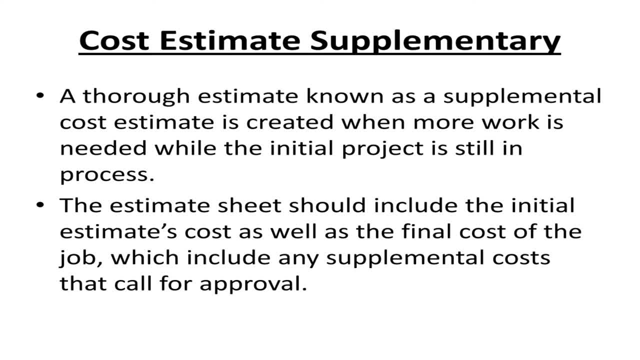 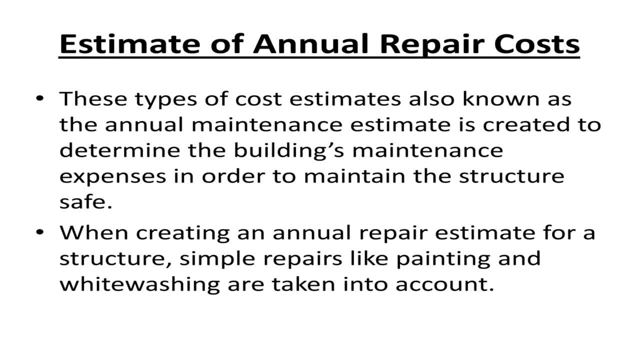 the estimate sheet should include the initial estimate's cost as well as the final cost of the job, which include any supplemental costs that call for approval. Estimate of annual repair costs. These types of cost estimates, also known as the annual maintenance estimate, is created to. 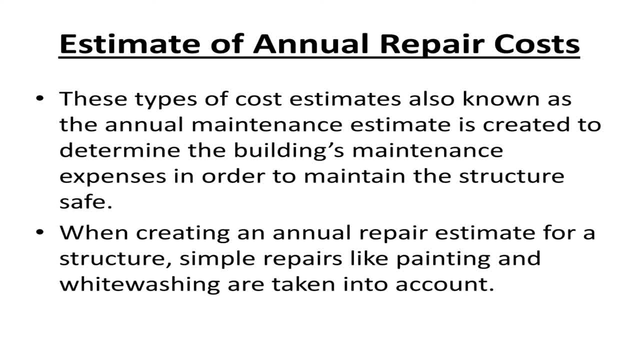 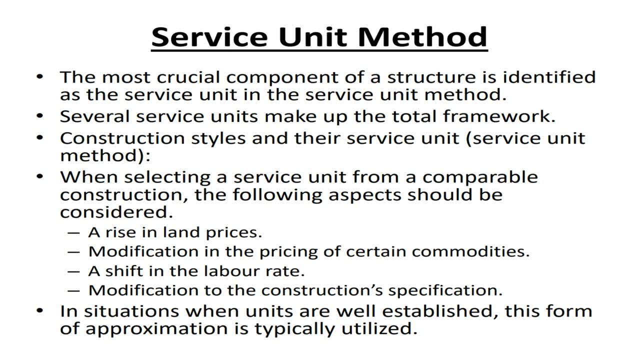 determine the building's maintenance expenses in order to maintain the structure safe. when creating an annual repair estimate For a structure, simple repairs like painting and whitewashing are taken into account. Service unit method: The most crucial component of a structure is identified as the service unit. 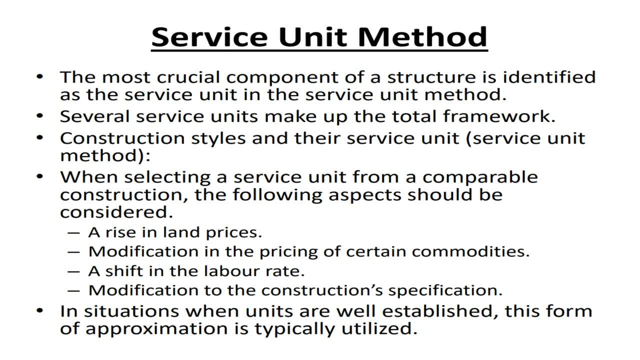 In the service unit method. several service units make up the total framework construction styles and their service unit Service unit method. When selecting a service unit from a comparable construction, the following aspects should be considered: A rise in land prices modification. 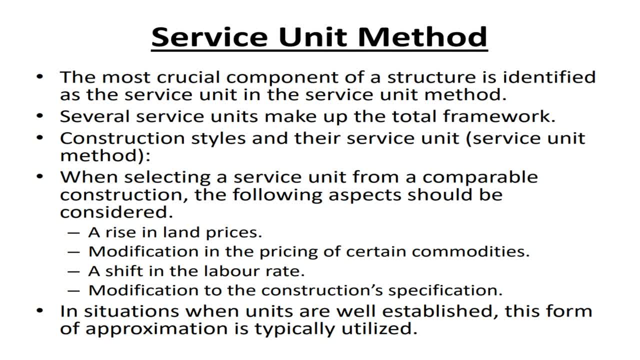 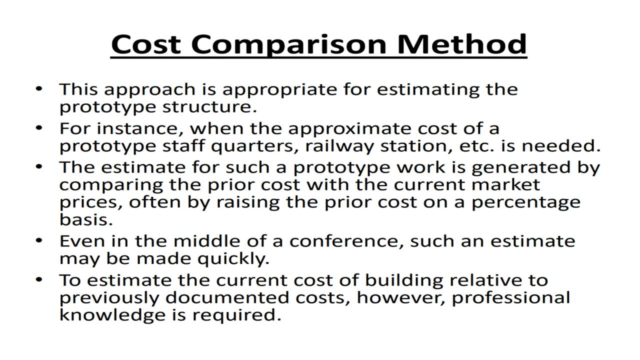 in the pricing of certain commodities, a shift in the labor rate, modification to the construction specification. In situations when units are well established, this form of approximation is typically utilized Cost comparison method. This approach is appropriate for estimating the prototype structure, For instance, when the approximate cost of a prototype staff 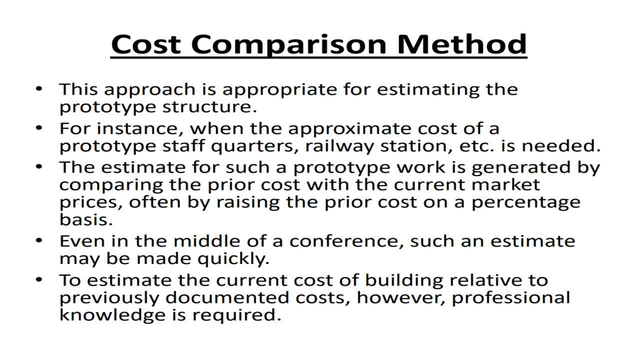 quarters, railway station etc. is needed. the estimate for such a prototype work is generated by comparing the prior cost with the current market prices, Often by raising the cost of the building on a percentage basis. even in the middle of a conference, such an estimate may be made. 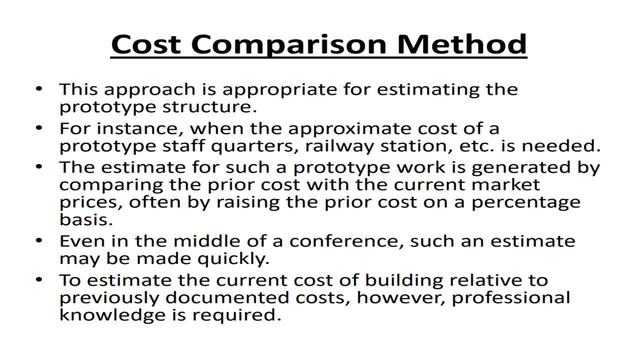 quickly to estimate the current cost of building relative to previously documented costs. However, professional knowledge is required.